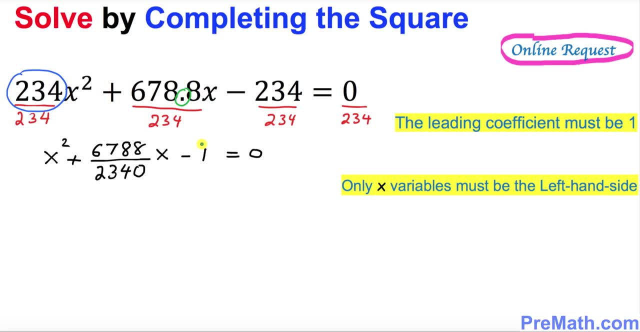 variables must be on the left hand side. That means this negative one must go on the other side. So we can write as: x squared plus six, seven, eight, eight, divided by two, three, four, zero, x equals to: when you move this negative one, the other side becomes positive one. 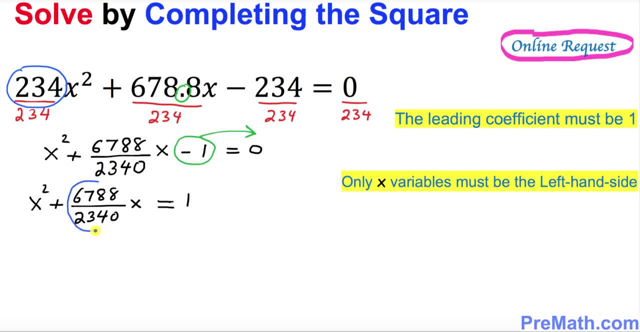 In the next step. I want you to just focus on this coefficient of x, Only this part. Don't worry about this sign. I want you to just put down this: whatever this quantity- six, seven, eight, eight divided by two, three, four, zero, whatever this amount is- I want you to divide this quantity by two. Dividing this one by two is same as: 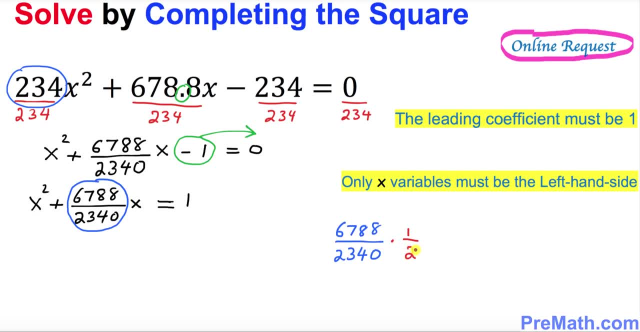 multiplying by one over two. All right, Now let's go ahead and simplify this thing. This two divides into this thing, as how much That's going to become? thirty three, ninety four. That means we simply got this thing. When you simplify this thing, this turns out to be thirty three, ninety. 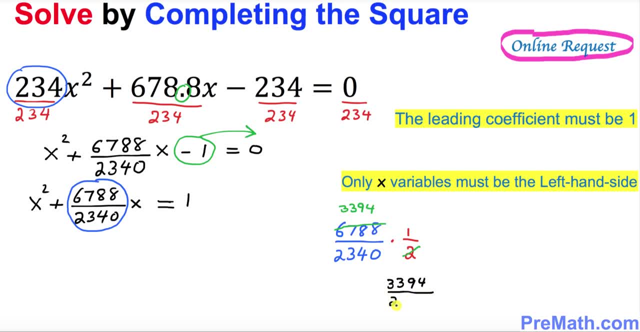 four divided by twenty, three, forty. Once we simplify this thing, the next step is: whatever this quantity you got, you must square this quantity, and whatever this quantity is, you must add on both sides of this equation. So let's go ahead and do that part. 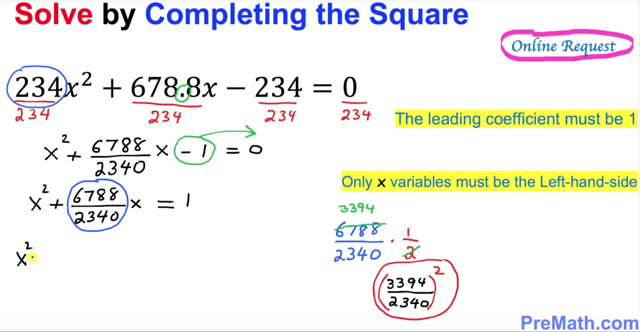 So let's go ahead and write down: x squared plus plus plus six, seven, eight, eight. divided by two, three, four, zero, x plus equals to one plus. what that means is now we're going to go ahead and add this quantity on both sides. that means i'm going to add: 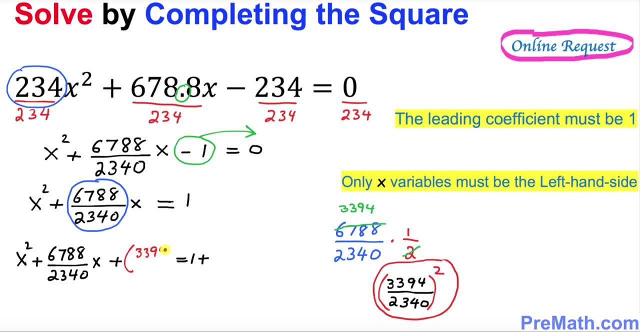 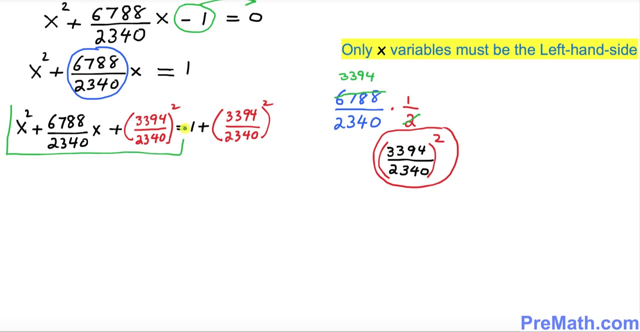 33, 94 divided by two, three, four, zero square on this side, and same quantity, 33, 94 over 23, 40 square on both sides. now i want you to look at, on the left hand side over here, this part, only this one, on the left hand side. this represents a complete. 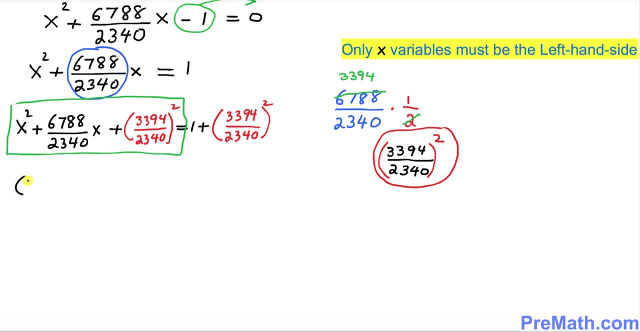 square of x plus 33, 94 over 23, 40 square, equals to this one. one could be written as, since we are dealing with the fractions, i can write one as a one over one. plus this, the square of the fraction is same as i can write the square of each part. i'm going to write: 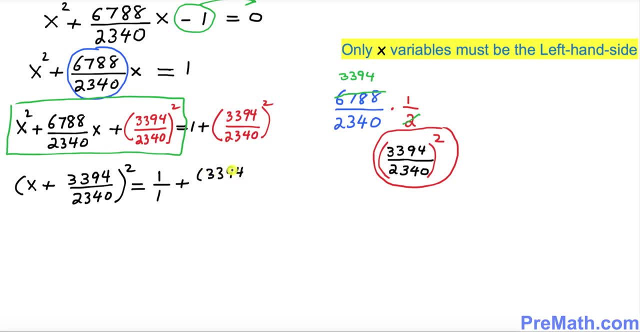 down: 33, 94 square divided by 23, 40 square. now if you are wondering how did we get this from this point, this step to this one, how we completed this square, we use this well-known fact: a squared plus two times a, b plus b squared could be written as a complete square of a plus b power. 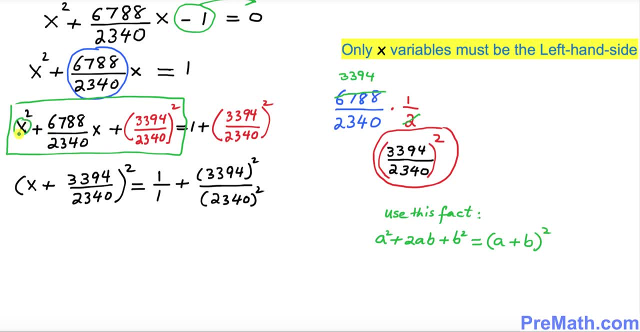 two. this is what i did, so over here, x moved right up here, this one here. whatever this quantity inside the parentheses, it showed up right up here. and whatever this sign is, it showed up right up here. and whatever this sign is, it showed up right up here. and whatever this sign is, it showed up right up here. 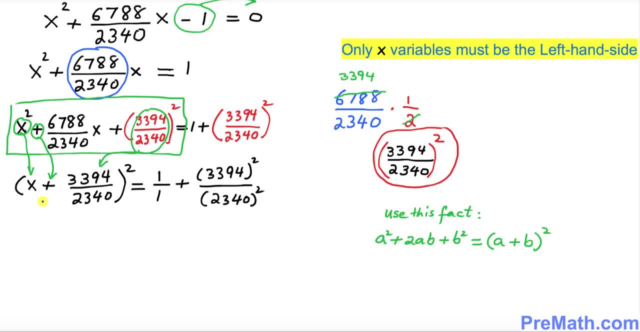 now let's go ahead and simplify further. let's go ahead and put it down this one i can write: x plus 33, 94 over 23, 40 square equals to: now we want to make sure that we should make the same common denominator. how are we going to make the same common denominator? 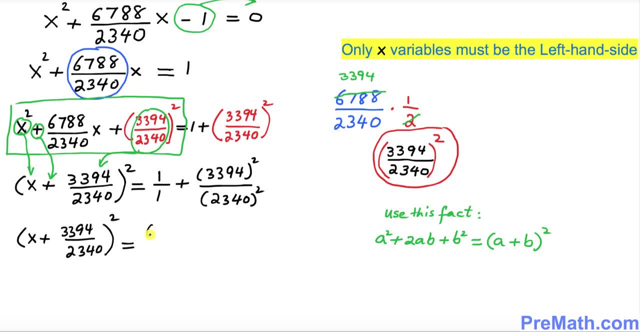 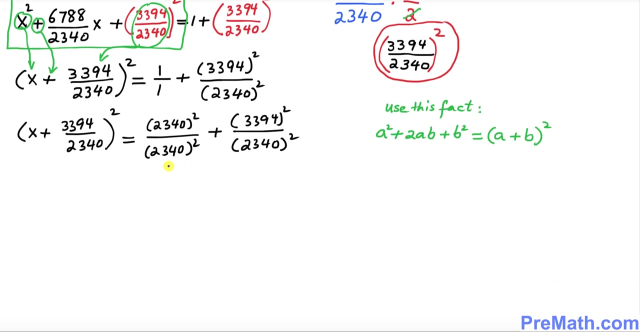 by just writing: 1 as 23, 40 square, divided by 23- 40 square, which is same as 1 plus, you can write this thing as same: 33, 94 square divided by 23- 40 square. so far, so good. since we got the same denominator- common denominators- we can write as simply: 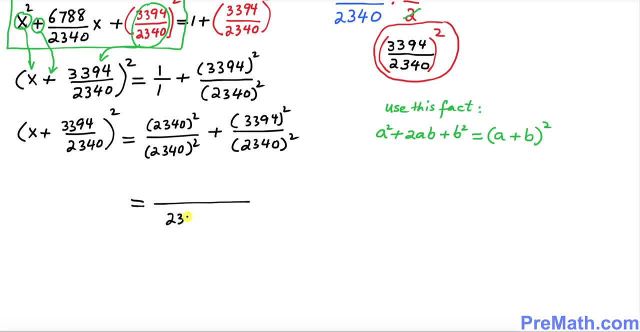 23, 40 square and on the right, on the top, is going to be on, the denominator is going to be 23, 40 square plus 33, 94 square and obviously on the left hand side is going to be x plus 33, 94 over 23, 40 square. now in the next step, if we use the calculator over here, i did the 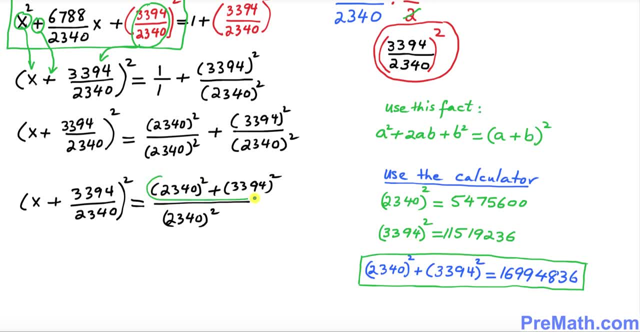 calculations over here, you can see that this quantity over here is same as this one over here, So I'm going to go ahead and replace that one. So I can write this one as 16994836 divided by. just leave that one as it is 2340 squared. 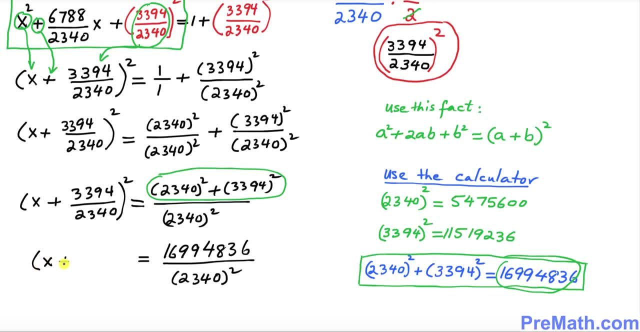 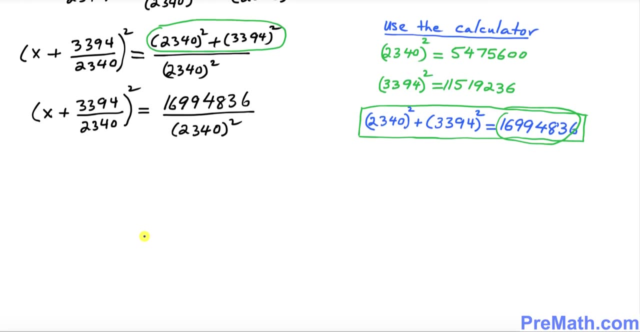 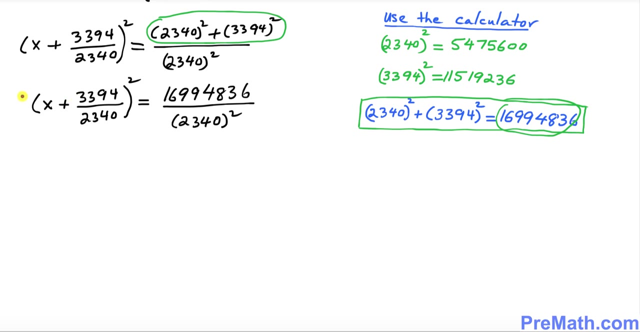 And obviously this is going to be x plus 3394 divided by 2340, whole square. So far, so good. Now the next thing: we want to isolate x. We want to get rid of this square, We want to undo this square. So we must take the square root on both sides. 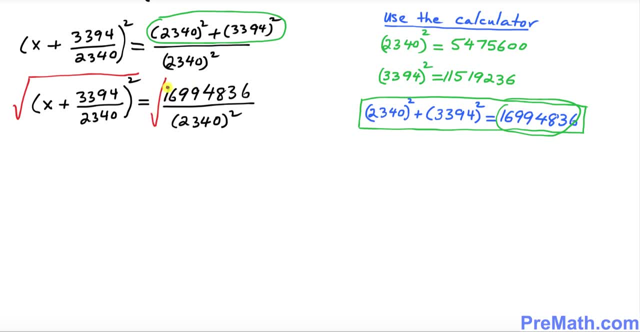 I'm going to take the square root on this side And I'm going to take the square root on this side as well. as you can see, this square and square root, they undo each other. we got x plus 33, 94 over 23. 40 equals to positive or negative. just keep in your mind. 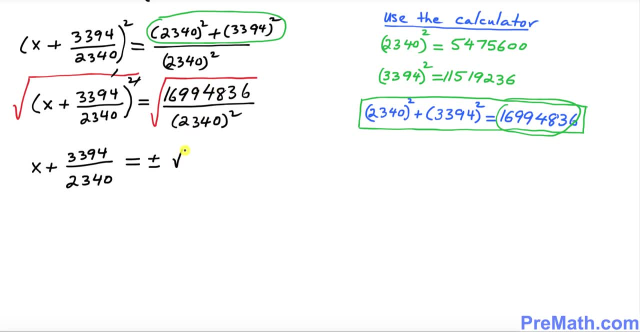 and here i can break it down. i can write as the square root on the top. i can just simply put down 16, 99, 48, 36, divided by the square root of 23, 40 square. all right, let's do the next step right now. 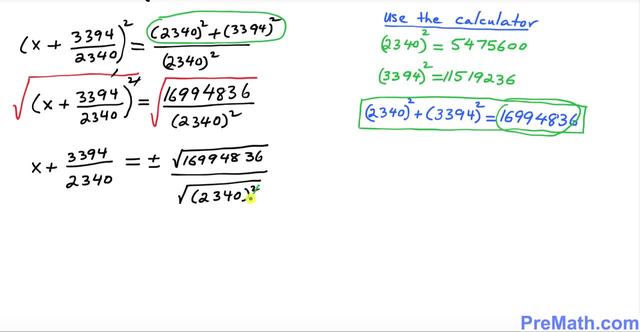 over here. as you can see, over here, this once again, this square and square root of 23, 40 square. all right, let's do the next step right now. over here, as you can see, square root, they undo each other, so let's go ahead and simplify further. we can write x plus. 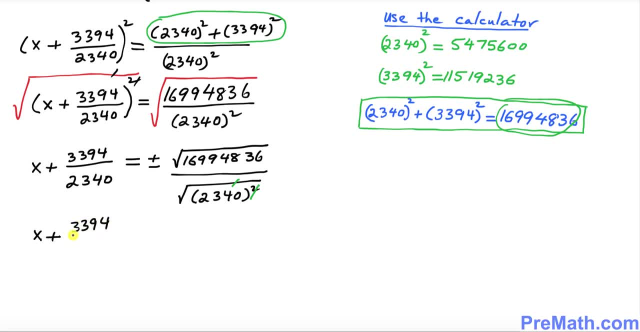 33, 94 divided by 23, 40 equals to positive or negative the top. when you take the square root of this quantity that is going to give you- i want you to use a calculator that's going to give you- 41, 22.48 divided by this thing, they both cancel out. so we got 23, 40. so far, so good. 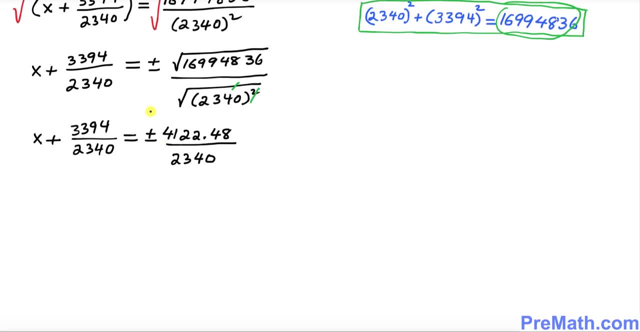 now the next step is: we want to isolate this x. so i want you to move this quantity on the right hand side. so once you move this thing on the right hand side, so we got x. equals to when you move this positive on the other side. this positive sign become negative. 33, 94 divided by 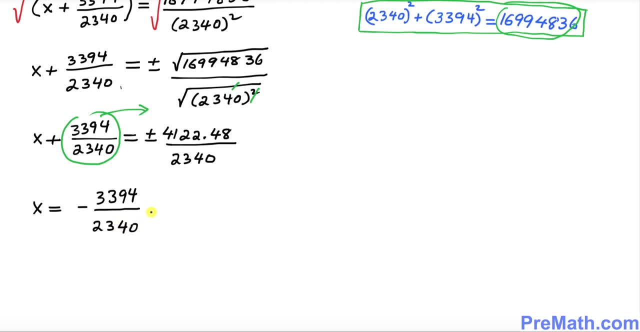 23: 40 positive or negative: 41, 22.48 over 23: 40. as you can see, we have the same denominator. i can write as i can write as negative. i can write this thing as the common denominator: 23: 40 over here, since the same. 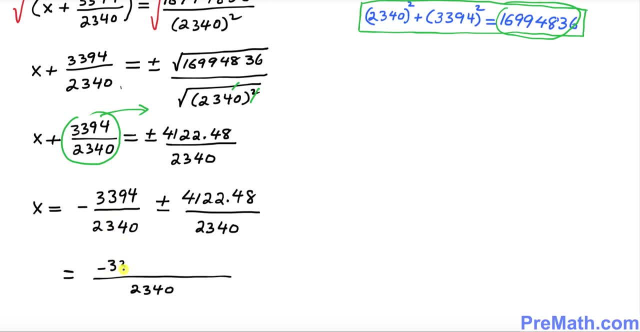 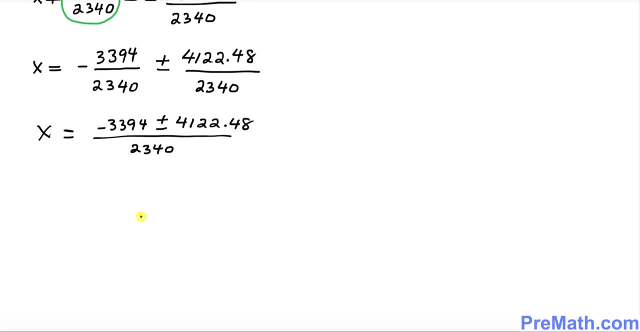 common denominator. i can write 30 negative, 33, 94 positive or negative, 41, 22.48, and this is equal to x. so our we are almost finished. let's go ahead and simplify this one. we're going to split this up along these positive and negative signs. so here: 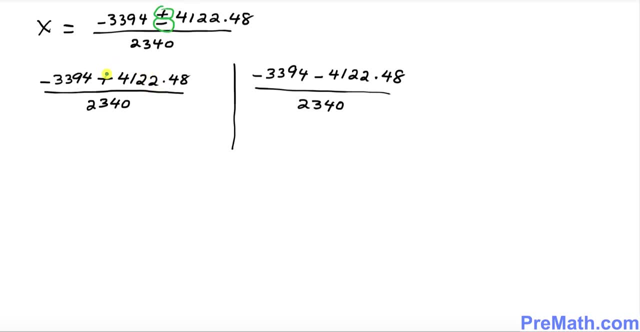 i have split, split them up, first with the positive sign right up, and then i'm going to split this up here, and then with the negative sign over here. let's go ahead and simplify this one, since these are positive, negative, unlike signs. so we're going to subtract, so that's going to give us. 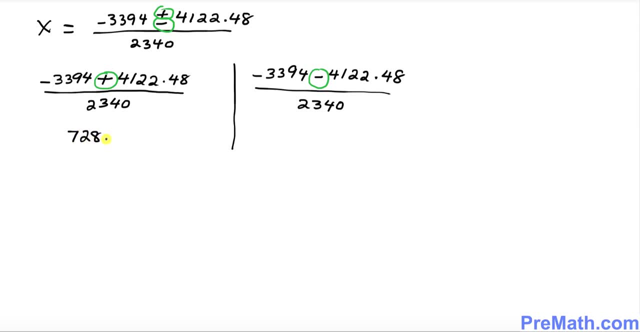 positive, 728.48 divided by 23, 40 and if you use the calculator, so this is product majority right equal to family eight, integral right equal to 12.20 and the赤 is equal to 216.. justice here. and we're going to divide and add that negative twice. that's going to give us 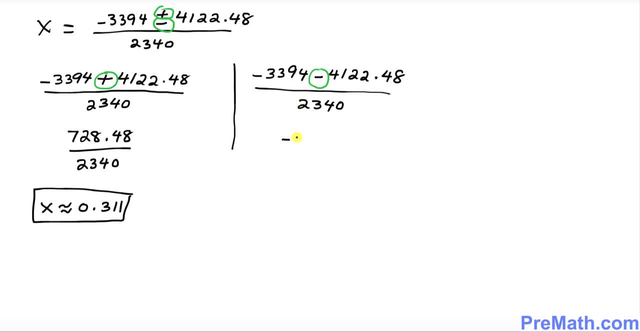 beads. here this is positive- will be the Loch gracias plus two. they're actually negative. 25 den彦 diva b, x is going to be approximately barely equal to zero. point three: one one. so this is one of our solutions, and over here, when we combine these one, we're going to add them. so this is going to be simply negative: 75, 16.48 divided by 23. çıkar. 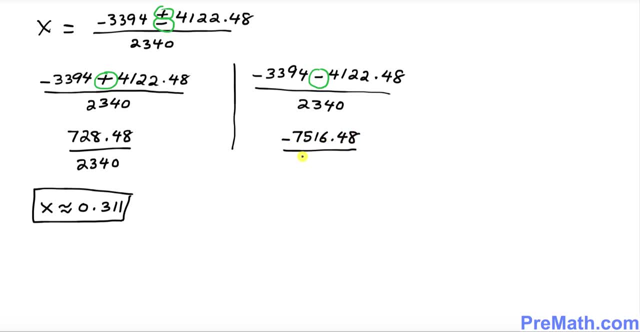 dis carter, den carter divided by 2340.. Once again, use the calculator and you're going to see this one that is going to become. x is approximately equal to negative 3.212. that is another solution. So thus, x is approximately equal to negative 3.212 and x is approximately equal to 0.311 are our two? 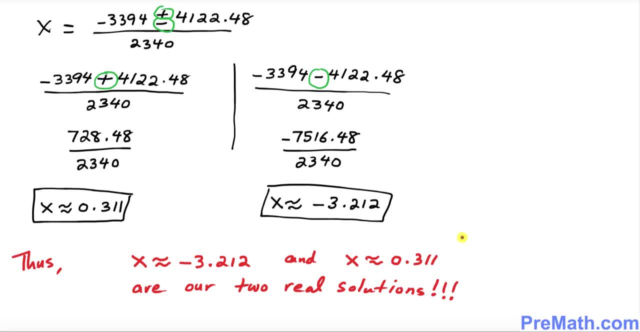 real solutions. Thanks for watching and please subscribe to my channel for more exciting videos.